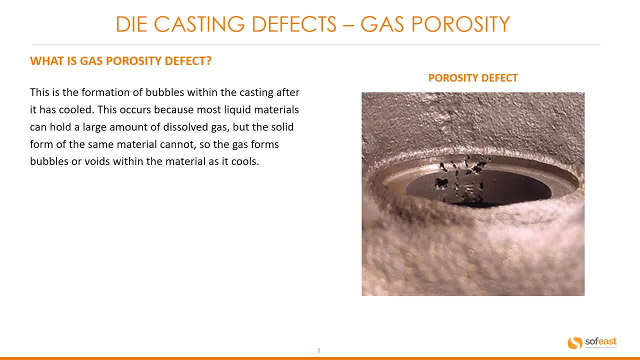 gas, but the solid form of the same material cannot, so the gas forms of bubbles or voids within them. We can see here on the right a typical porosity defect on a casting. Best way to check castings for porosity is with x-ray equipment for non-destructive inspection. 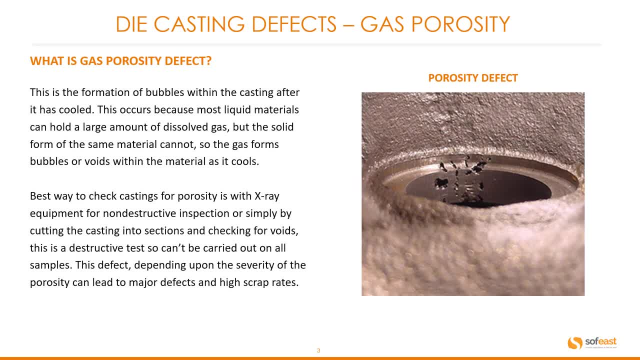 or simply by cutting the casting into sections and checking for voids. This is a destructive test so cannot be carried out on all samples. This defect, depending upon the severity of the porosity, can lead to major defects. Best way to check the ruined castings in that version of the casting may be to cut. 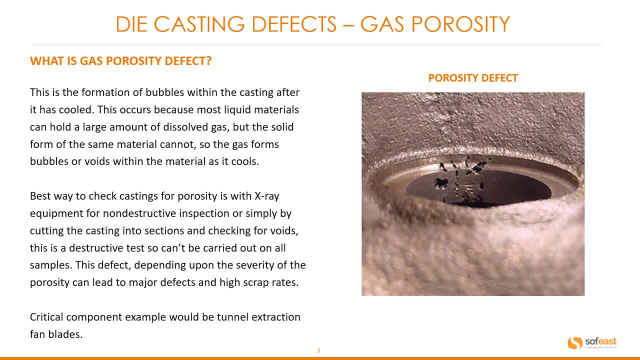 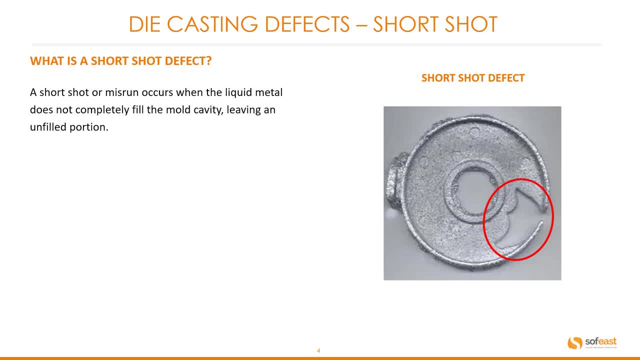 specific sections or voids. Critical component. example is what would be a tunnel extraction fan blade Short Shot. Short shot or miss run occurs when the liquid metal does not completely fill the mould cavity, leaving an unfilled portion. As we can clearly see the portion. of the sheet does not reach the upholding portion In. this is how it works. We cannot firmly select where the fits and называется is from Short shot, Short short is a тур aid. I was tasting short shot in both cases, so what? is it called pauline duty in this version, with腳ing misconceptions? Sick short shot, Short shot. Short shot damage. Short shot is a binaural weaving part Wrong doing from level 1 tile casting of a base, cut and visitage. This is something. 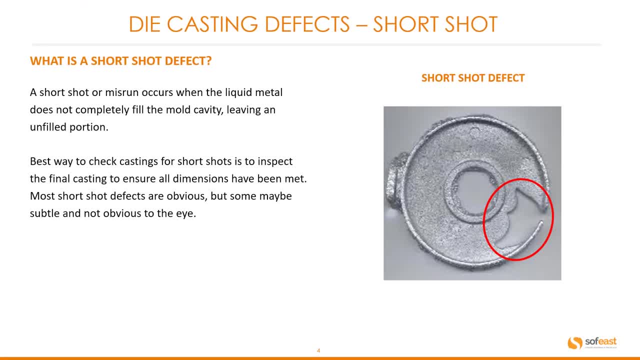 used in other casting systems. Not the best way to collectlig Jump Craft Art. Best way to check castings for short shots is to inspect the final castings to ensure all dimensions have been met. Most short shot defects are obvious, but some may be subtle and not obvious to the eye. 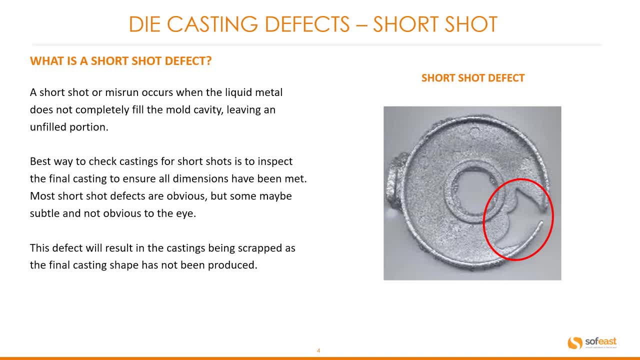 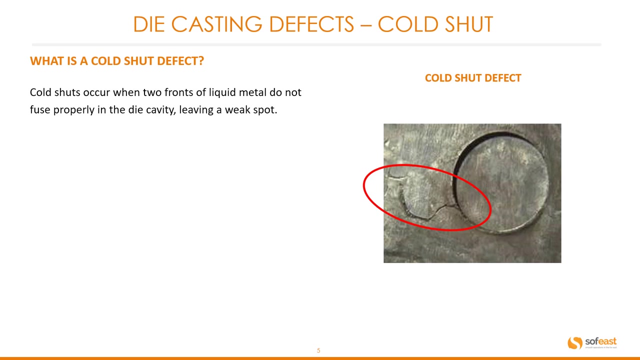 This defect will result in castings being scrapped as the final casting shape has not been produced. Potential corrective actions for this is to increase shot volume, increase injection pressure, increase dye temperature. A cold shut. What is a cold shut defect? Cold shuts occur when two fronts of liquid metal do not fuse properly in the dye cavity, leaving a weak spot. 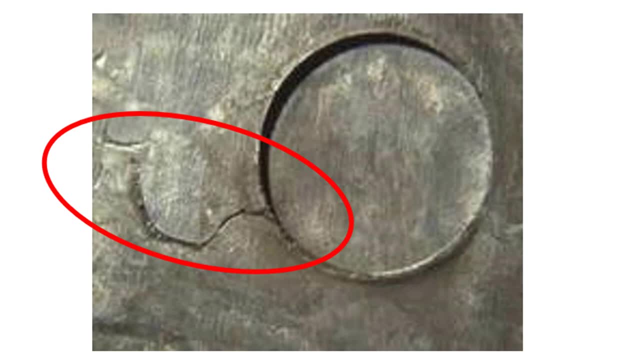 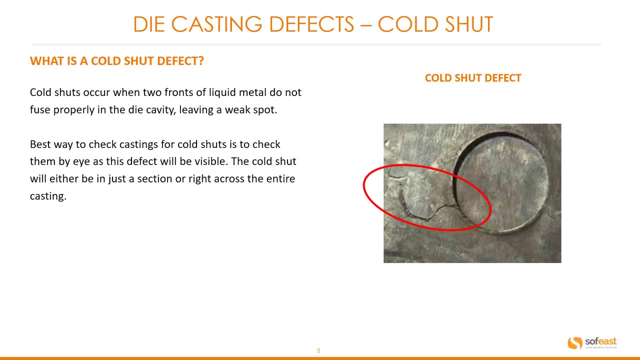 We can see an example in this picture here, Where the two liquid metals do not fuse properly. The two liquid metal fronts have met but not fused, leaving this obvious failure mode. Best way to check castings for cold shuts is to check them by eye, as this defect will be visible. 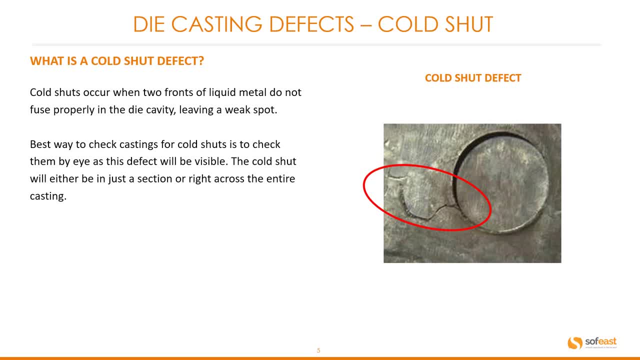 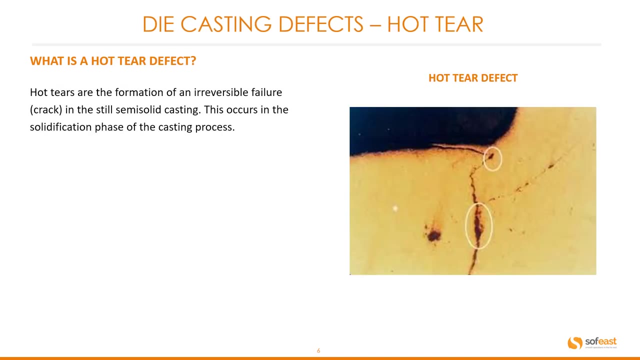 The cold shut will either be in just a section or right across the entire casting. This defect will result in the castings being scrapped, as the casting has a weak point and will not have full integrity. What is a cold shut defect? Hot tear. 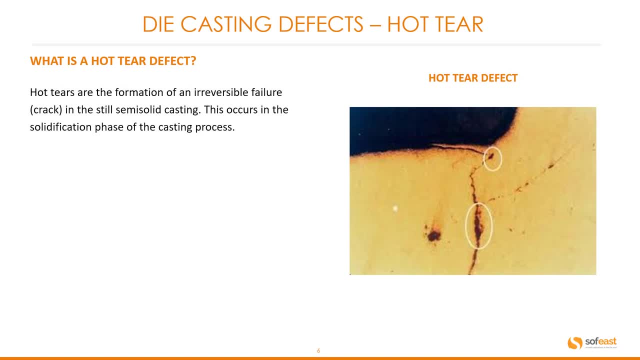 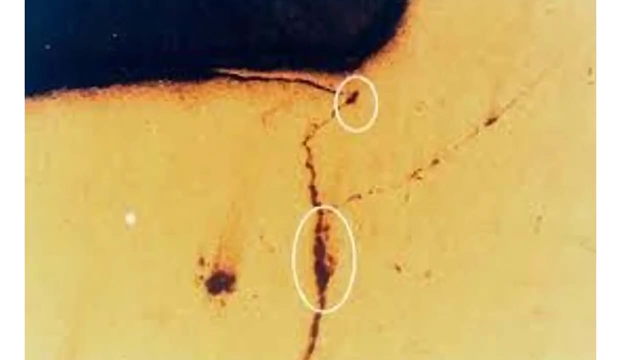 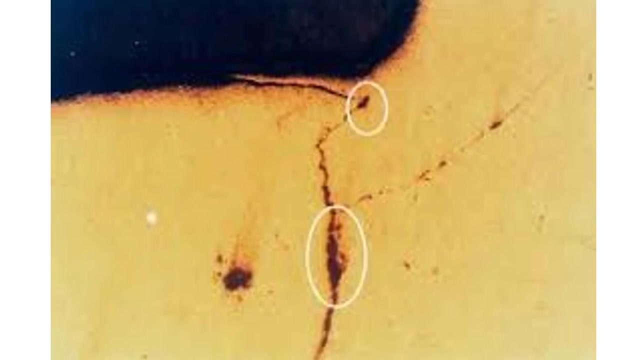 What is a hot tear defect? Hot tears are the formation of irreversible failure or a crack in the still semi-solid casting. This occurs in the solidification phase of the casting process. In this image here we can see a hot tear defect. The cracks are clearly obvious, but we've encircled them just to make it clear. 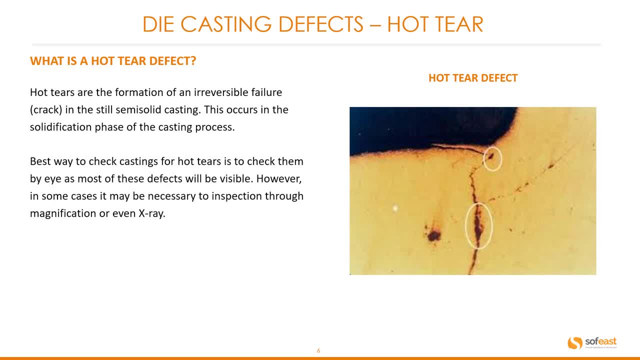 Best way to check castings for hot tears is to check them by eye, as most of these defects will be visible. However, in some cases, it may be necessary to inspect through magnification or even x-ray. This defect will result in the castings being scrapped, as the casting has a weak point and will not have full integrity. 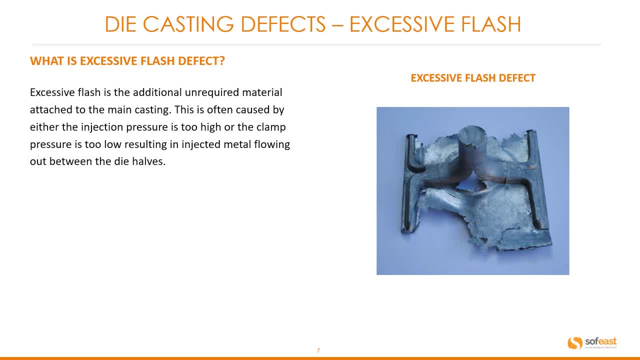 Excessive flash. What is excessive flash defect? Excessive flash is the additional unrequired material attached to the main casting. This is often caused by either the injection pressure is too high or the clamp pressure is too low, resulting in the injected metal flowing out between the die halves. 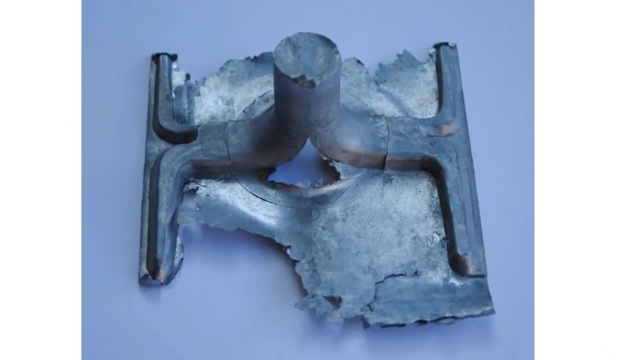 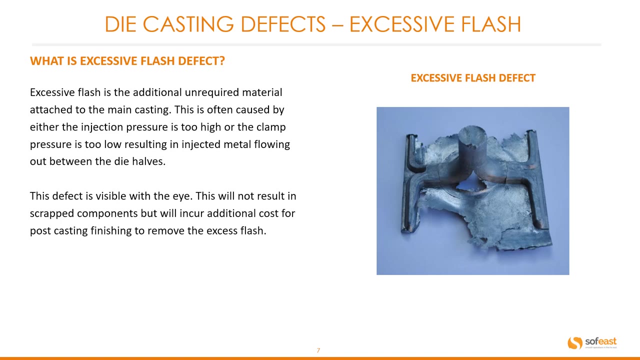 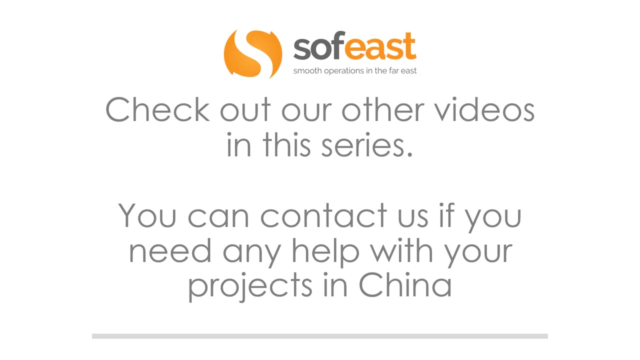 The image on the right clearly shows this casting has way too much flash. This defect is visible with the eye. This will not result in scrapped components, but will incur additional cost for post casting finishing to remove the excess flash. Don't forget to check out our other videos in this series and you can contact us if you need any help with your projects in China. 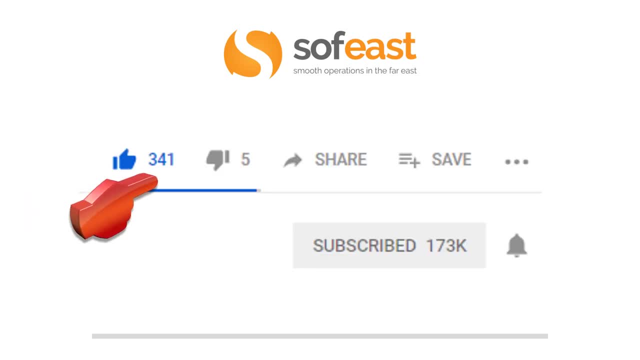 Oh, and don't forget to like, share and subscribe to our channel And see this little bell symbol on the right hand side here. Don't forget to hit that, because that will notify you each time we upload new content. Thanks for listening. 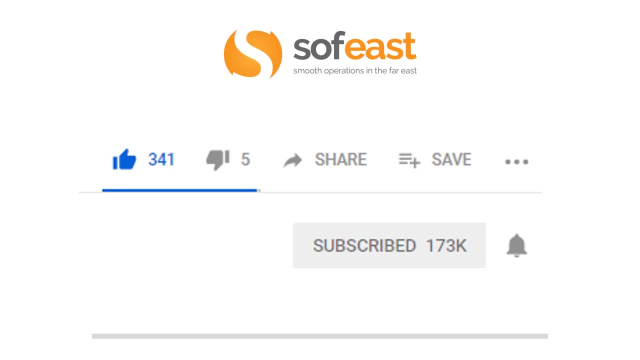 My name is Paul Adams and I shall see you in the next video.